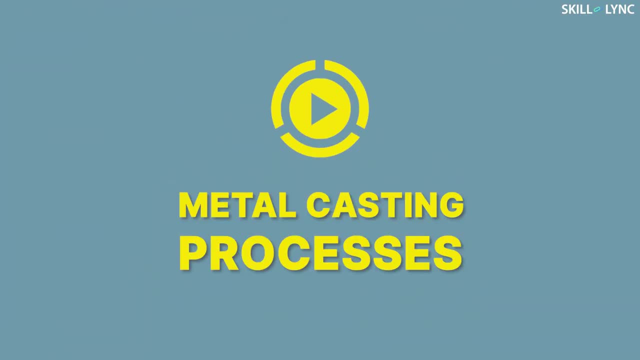 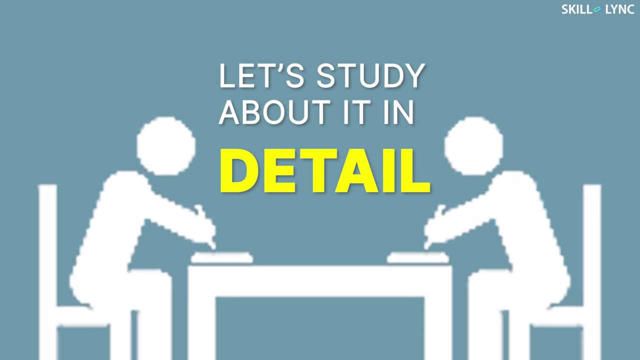 around 3200 BC. In today's video, we will talk about one of these metal casting processes, that is, sand casting. Sand casting is the most widely used casting process. Let's study about it in detail, shall we? First of all, let's discuss the casting process. What exactly is meant by? 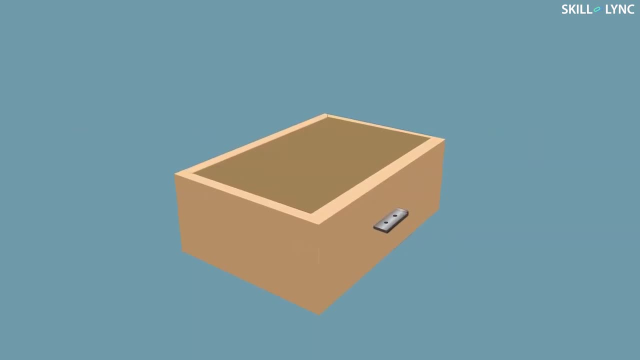 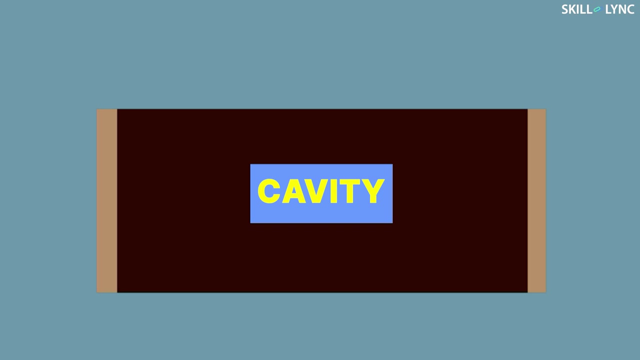 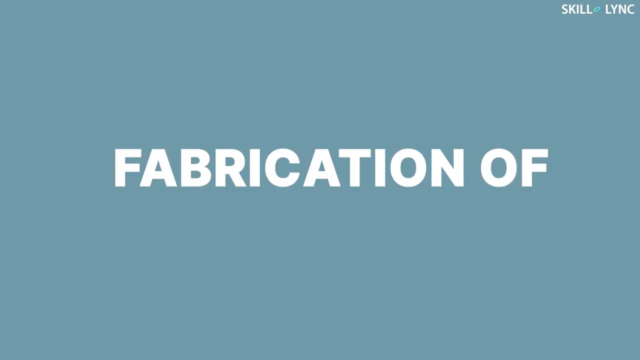 casting process. Well casting is a manufacturing process in which molten metal is transported into a mold and allowed to cool down. This mold has a cavity of the desired shape. As the molten metal cools down, it solidifies and takes the shape of the cavity. This process is used for the 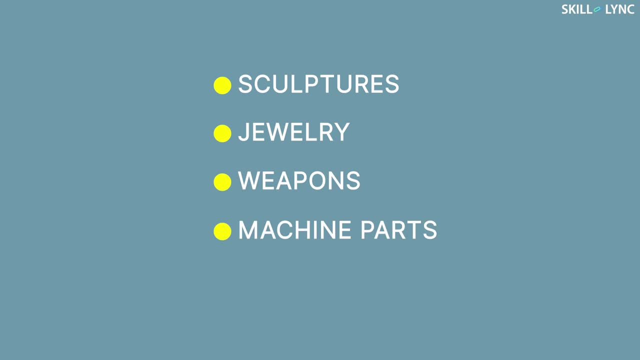 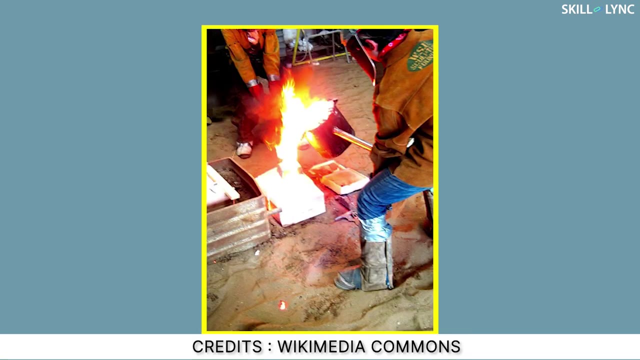 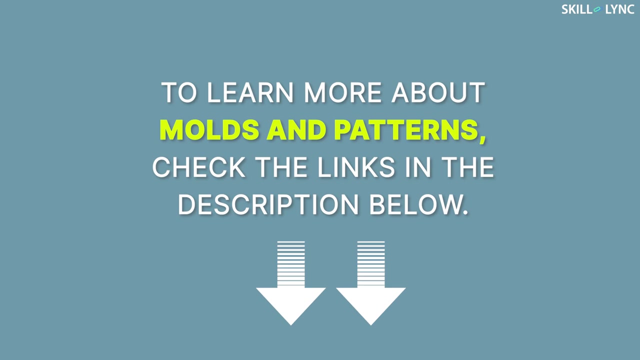 fabrication of sculptures, jewelry, weapons, machine parts, tools, etc. Sand casting is perhaps one of the most popular and simplest casting process. Just as the name suggests, sand casting employs expendable sand molds to manufacture complex parts. For this process, a furnace is. 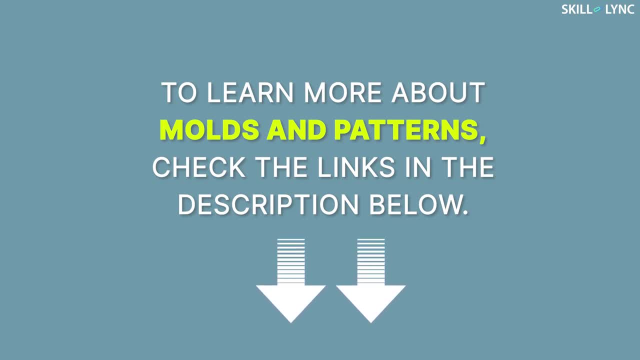 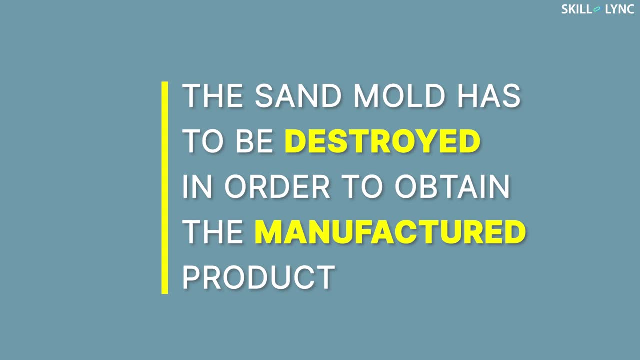 required to be casted into a mold and allowed to cool down. This mold has a cavity of the desired shape. along with the molten metal, sand mold and pattern Sand casting has a low productivity rate. This is because the sand mold has to be destroyed in order to obtain the manufactured product. 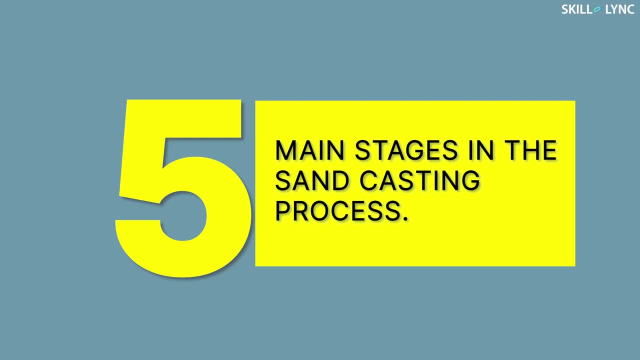 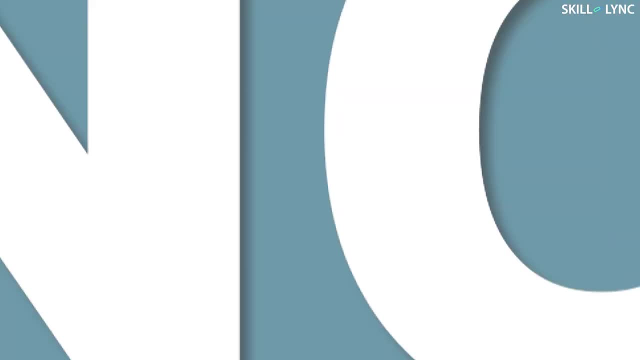 Let's discuss the method of sand casting in detail. There are five main stages in the sand casting process. What do you guys think about? the first stage Is obtaining molten metal. the first stage? Well, the answer is no. The first stage of the sand casting process is the creation of sand. 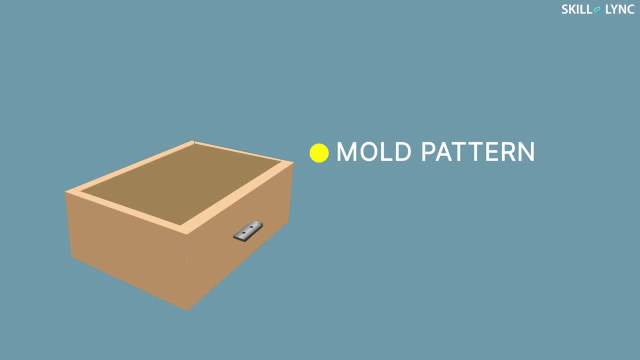 mold. As you can see in the animation, we take two halves of the molten metal sand mold and pattern. One half of the pattern is placed on the surface of one box. Sand is poured into this box and a pressure is applied for tightly packing the pattern into the sand. After this, the box is inverted and 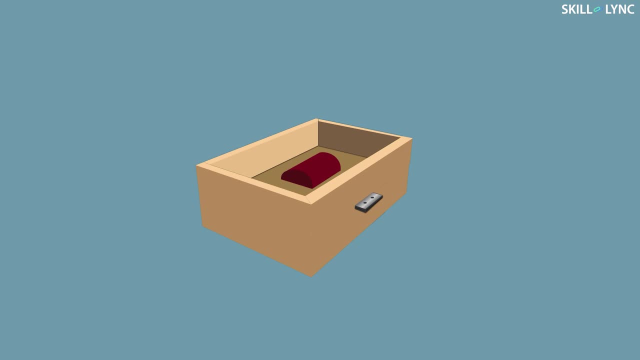 the second box is placed on it, The other half of the pattern is placed exactly on top of the first half, and then sand is poured. Once again, we apply pressure on the boxes so that the pattern gets tightly packed with the sand. Now the boxes are opened and the patterns are removed with the help. 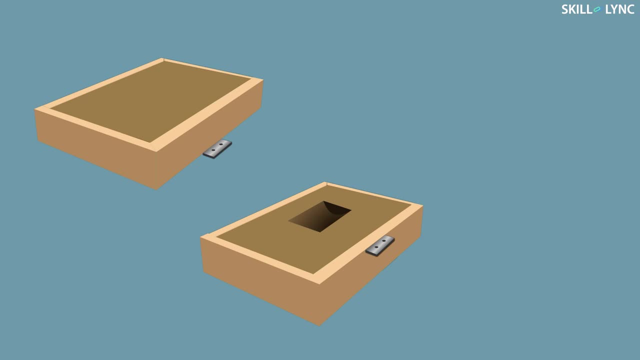 of screws. Hence the mold is casted into the sand. The second half of the pattern is placed on top of the first half of the sand. The mold has been created. After the mold has been created, it is prepared for further process. This is done by putting the boxes together again and clamping. 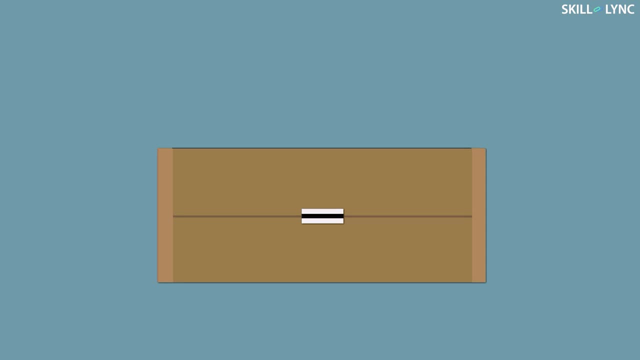 them with rivets. Clamping is done to prevent the upper box from floating over the lower box. What happens after clamping? Yes, we pour the molten metal. now, With the help of a furnace, the molten metal is obtained. This molten metal is then poured into the mold with the help of gates and 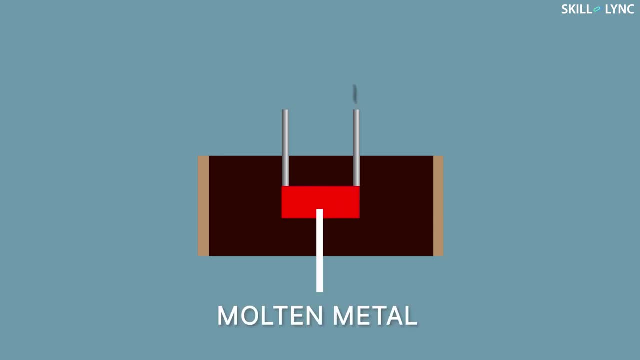 spruces. To avoid early solidification, the molten metal must be poured quickly. Once the molten metal is poured inside the mold cavity, the mold is ready to be casted. The mold is then casted into the. the mold metal is allowed to cool down. As a result, the molten metal solidifies. 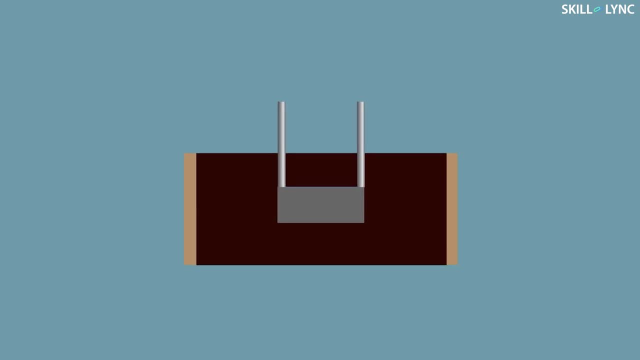 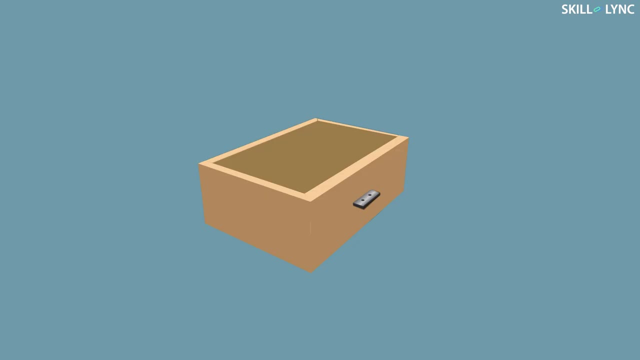 and takes the shape of the mold cavity. The time taken for proper solidification of the metal depends upon the wall thickness of the casting and temperature of the metal. Once the cooling stage is finished, the sand mold is broken and the casting is removed. After this, the casting is cleared and trimmed in order. 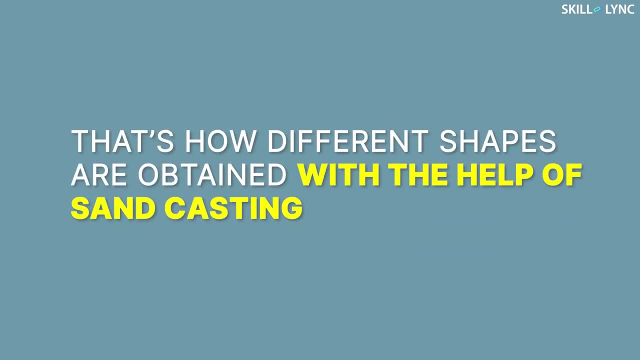 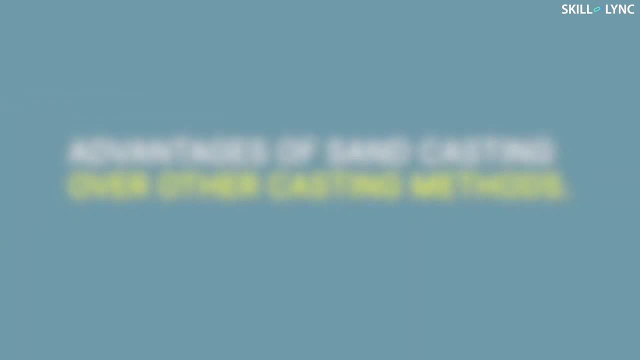 to remove any unwanted layer of metal. That's how different shapes are obtained with the help of sand casting. However, did you guys wonder why sand casting is the most popular casting process? Well, this is because of the advantages of sand casting over other casting methods. Also, the tooling cost of this process is 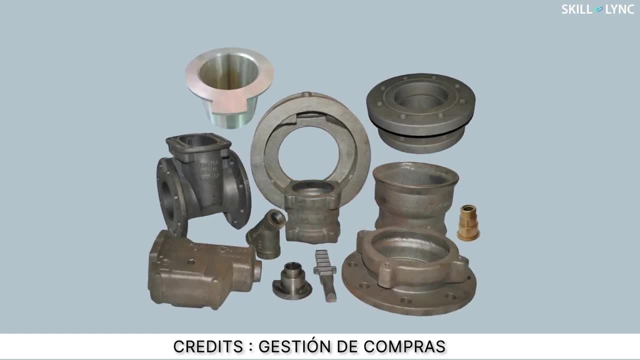 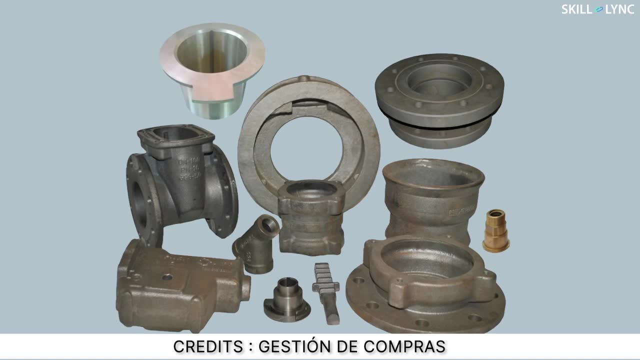 low, and the time taken during this process is lower. when compared with other casting methods, Sand casting process is versatile and hence a wide range of materials can be manufactured using this process. However, we all know that after the light comes the darkness, don't we? Well, sand casting is no. 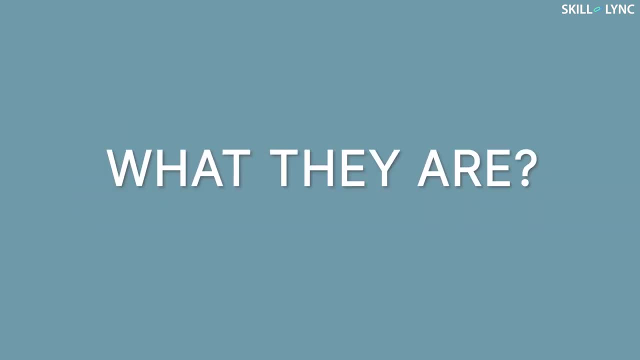 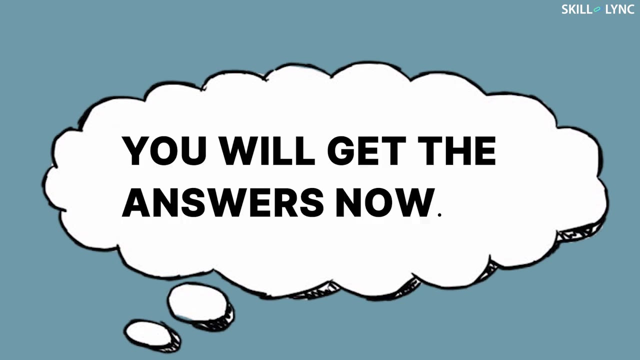 exception. There are a few limitations of sand casting. Wondering what they are? What do you guys think? Think about the dimensional accuracy and surface finish of the final product in this process. Well, you'll get the answers now. As you can see in this image, the sand casting. 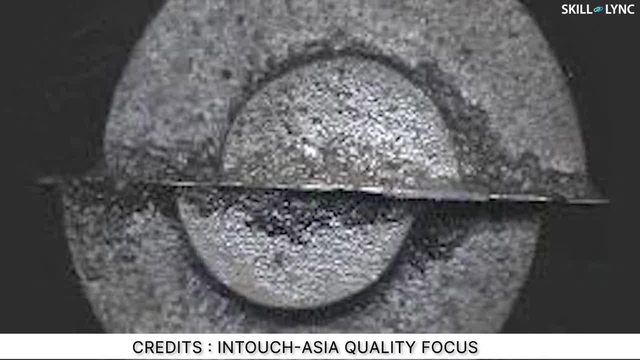 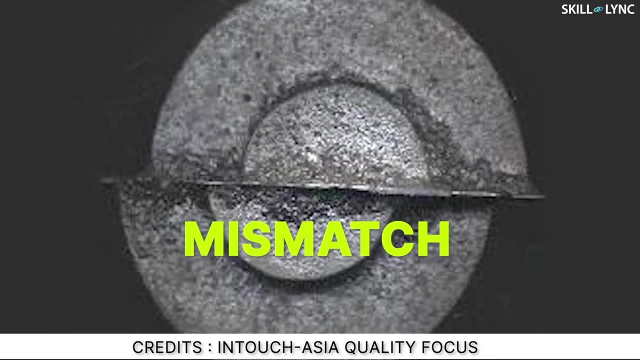 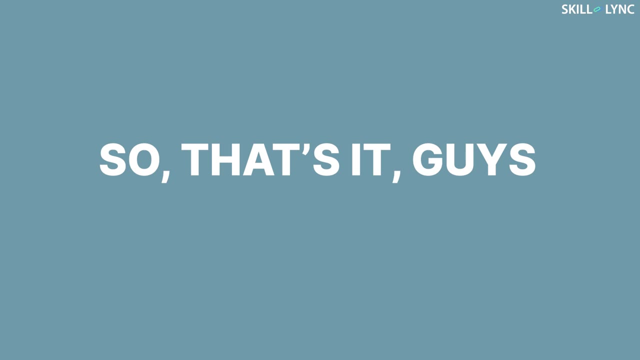 process suffers from a lower dimensional accuracy when compared to other casting methods. The surface finish is also not very good and requires proper trimming and chipping of the final product. On top of these, a proper maintenance of the mold pattern is essential. Well, that's all for today, guys. We'll be back with more content based on casting processes. 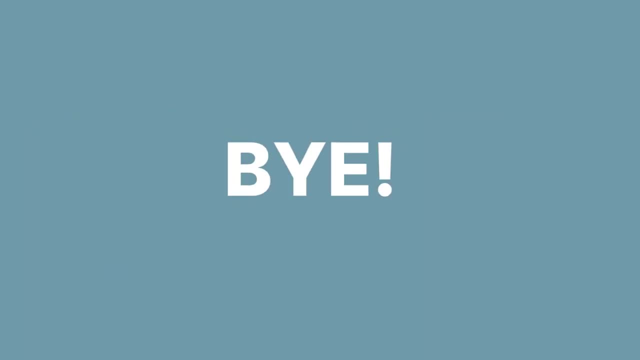 very soon. Stay tuned and stay safe Until the next one. bye.